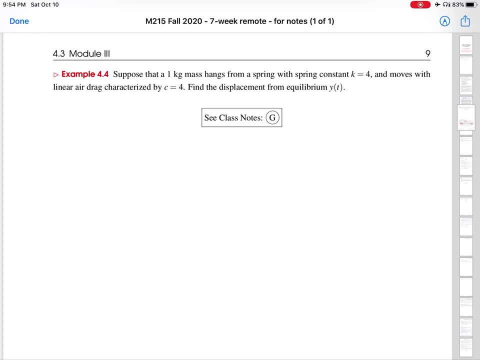 Hi, this is Professor Fernandez. Let's talk about class notes G from lesson four. So in this example we are considering a mass, one kilogram mass, that hangs from a spring with a spring constant K equals four, And I'm calling it here linear air drag. Again, that's the same drag force, air resistance, dashpot, all the same model that we've been using in this lesson, with C equals four, And the idea is to find the 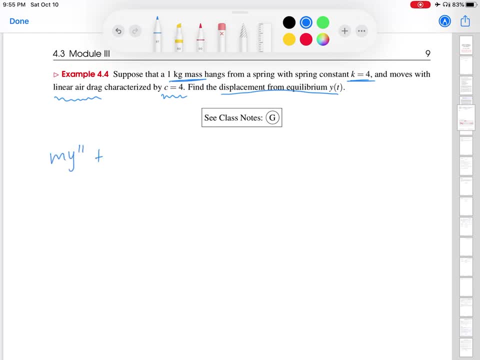 displacement from equilibrium. So I'm going to use the same model that we have been working with in this lesson And I'm just going to put in all the parameters. So I have that M equals one. I have C equals four. Again, I'm sort of ignoring the units and assuming they're all SI. And then K equals four as well, And then characteristic equation here: replace the orders of the derivative with powers of R. So I get that. 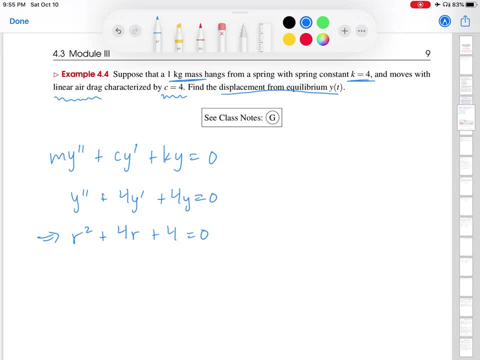 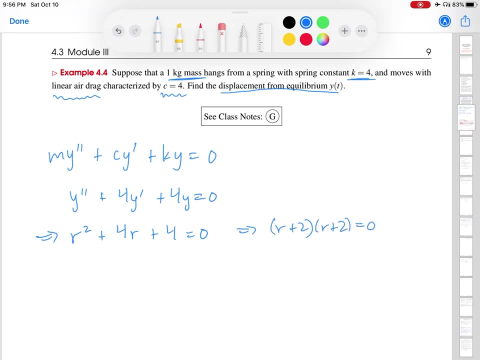 that's- And I'm going to try to factor here, but see how it works, How about we try R plus two, R plus two, And we'll double check that. So R squared plus two, R plus two, R, that's four, R plus four. So that seems to work. So this is going to give us a repeated root. We are going to get R equals negative two and also negative two. So we are in the case that we just 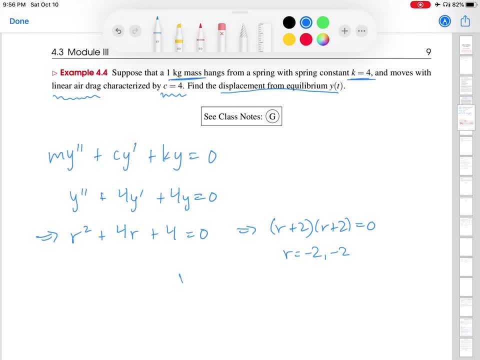 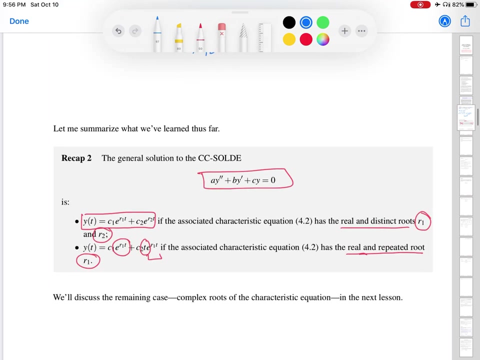 in the previous video in this lesson. So you know you might think: oh so I have the two solutions, e to the minus two t and e to the minus two t, And while that's true, these two solutions do not form a fundamental set of solutions because they're Ronskin zero. So we talked about in the previous video how what we're doing- and that's you know, down here, left over from those markings- What we're doing is that we now have a real repeated root, In this case negative two.